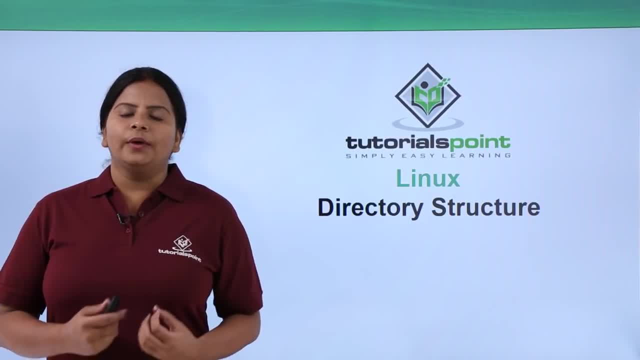 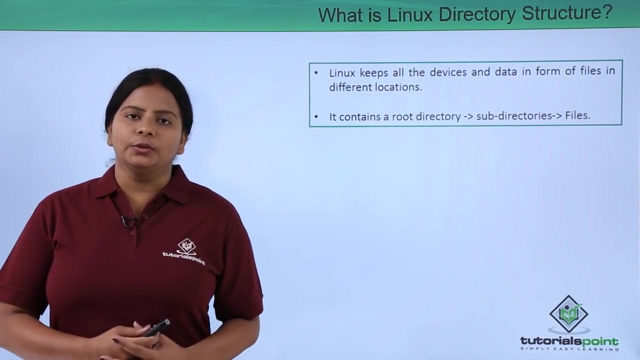 completely open-source, so you can see everything- value generally, devices, your programs, your configurations are stored. so here we are going to talk about your Linux directory structures. so let's, directory structures generally stores the data into completely different locations, unlike your windows, so here everything is stored as an file and folders. 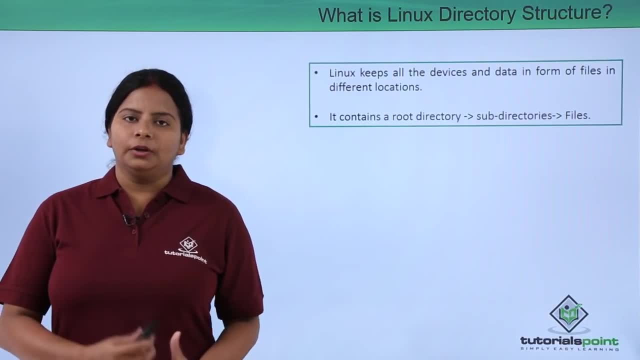 you use it for everything. here you are able to store your files and you can keep. even your devices are stored into the files in a particular folders, so the folders has multiple sub directories, sub folders into that. you also keep some of the files. so basically you should understand what this folder contains. 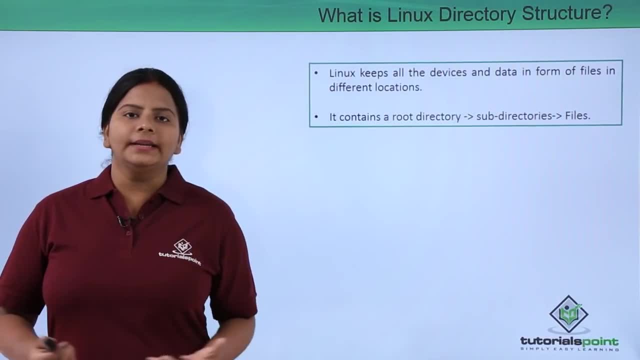 because when you install the operating system you won't find any c drive, d drive, e drive or your my computer, but everything you will find, that is your slash, which is called as front slash, or a mount point. under that one point you will find a different directories which we are going to see over here. we'll 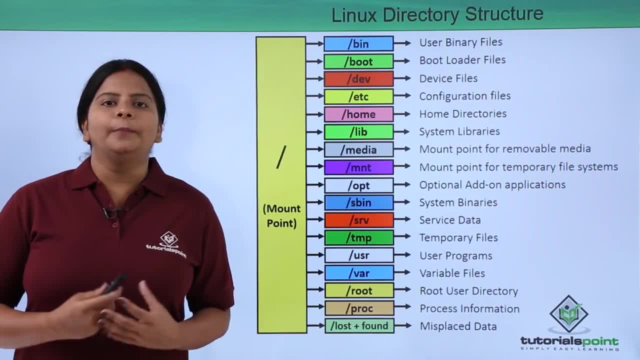 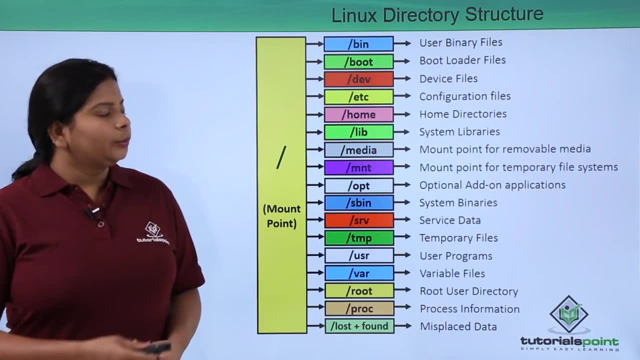 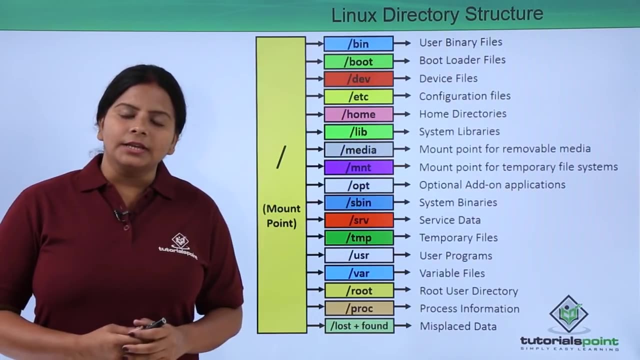 find a directory called as slash bin. slash bin is a binary files, so whatever the commands you are going to store will be located into the binary file, and all these directories which you can see here are generally created into the mount point which is your front slash. so this mount point contains all the particular directory. 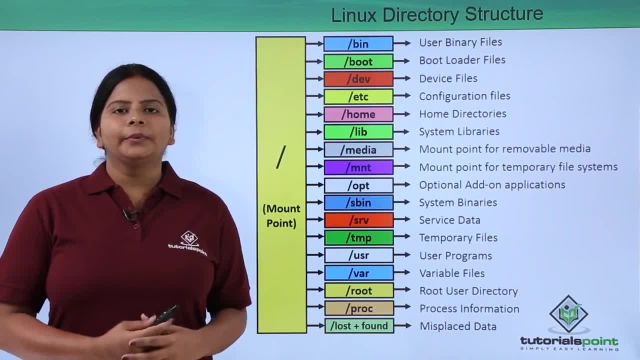 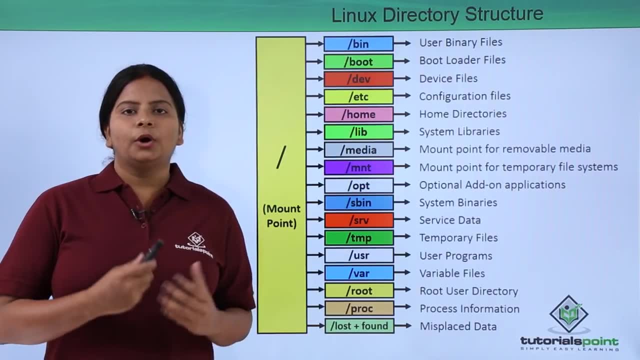 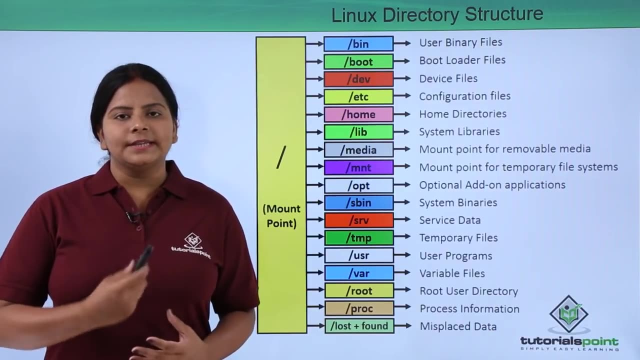 each and every directory you can see over here contains different tasks and contains different contents. so very first, we are going to talk about slash bin. so whatever the command generally you have or you generally use, like creating a user, creating a file, creating a directory, everything will be stored into this slash. 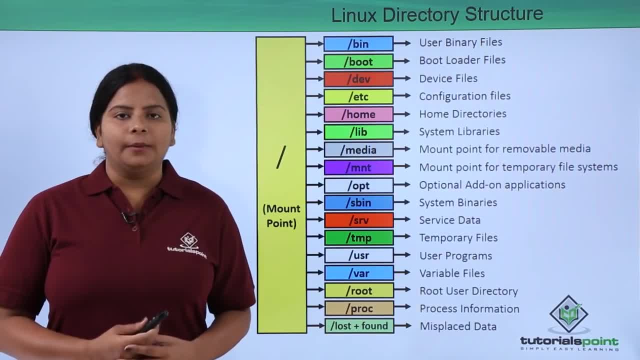 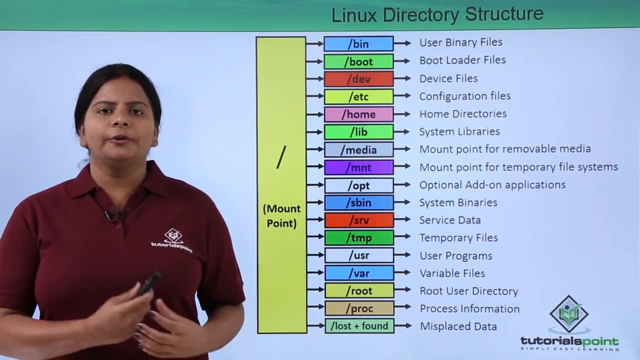 bin, which contains all the files for your complete commands. so basically, when you run the command this, binary files get worked and it provides you the output. the next we have the output of the binary files which we have, that is, slash boot. so, like your windows operating system, you might have seen some system reserved. 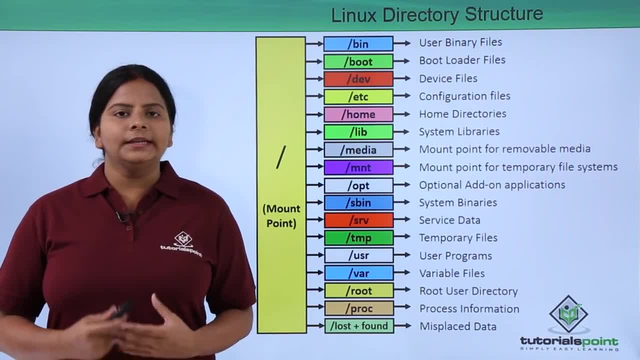 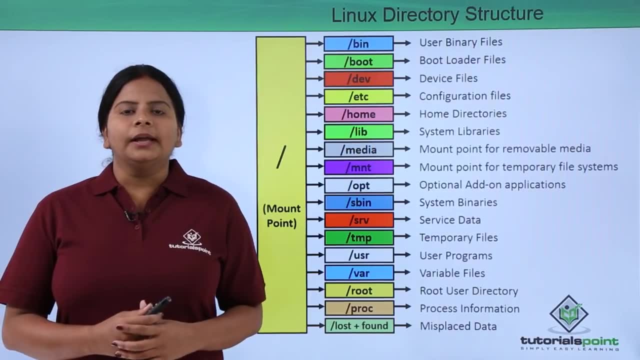 partitions into the operating systems. like your windows 7 contains that, your windows 8 contains it, as well as tense container. so what the system reserve partition is? it contains your booting file. same here in the linux operating system. we have all the booting files installed. 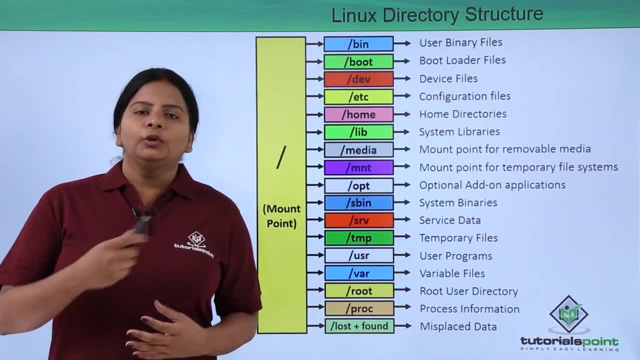 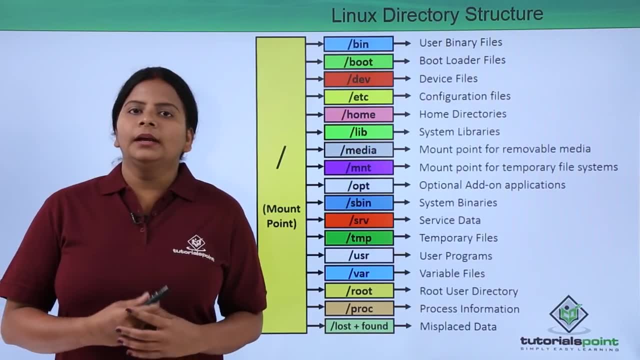 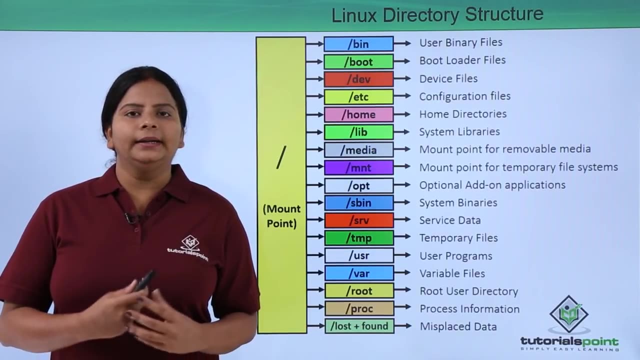 into this particular directory by default. so when you install the linux operating system you will find the booting files as your boot, and here the booting file is completely different. here you will find grub or grub 2 as your booting file, and in earlier version of your linux operating system you used to also find 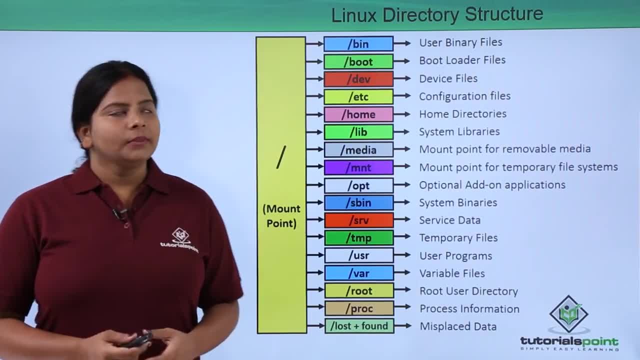 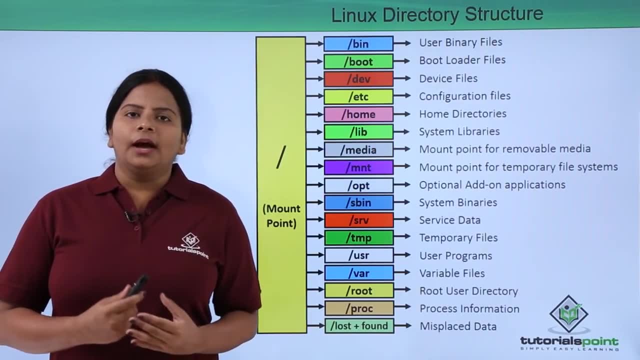 lilo operating systems, which we are going to discuss later. the third file which we have, that is your slash tape. this directory contains all the devices files like if you have connected your hard disk, if you have created a partition into the hard disk, everything will be stored into devices. if 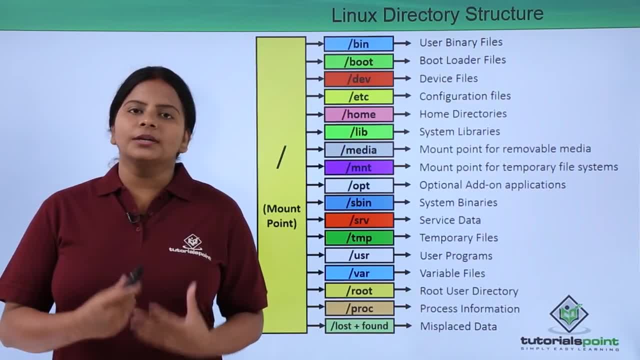 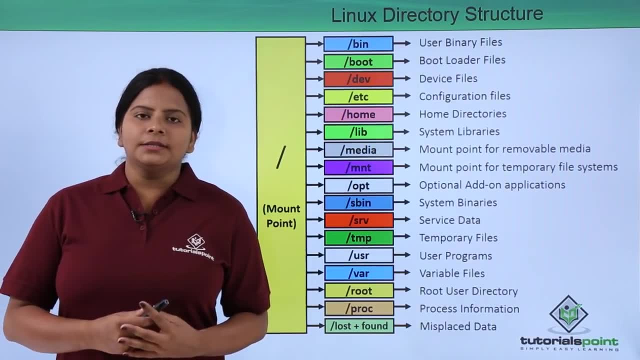 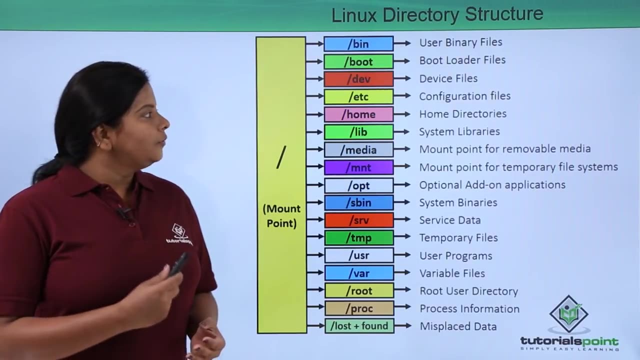 you have connected to any particular usb drive. if you'd use a dvd drive or cd drive, this will again be stored into the devices. so whichever the device you connect- either it isn't directly attached devices or a removable or hot plug-in play devices- all will be stored into slash tape. next we have that is slash, etc. 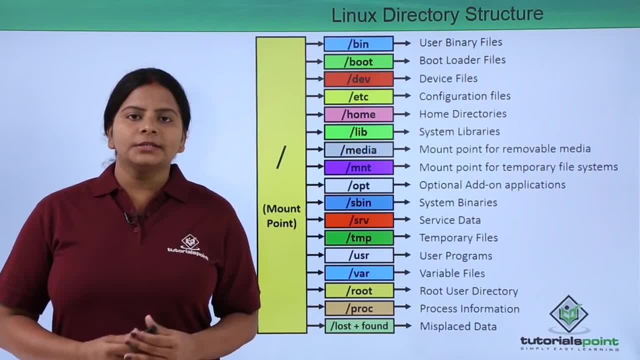 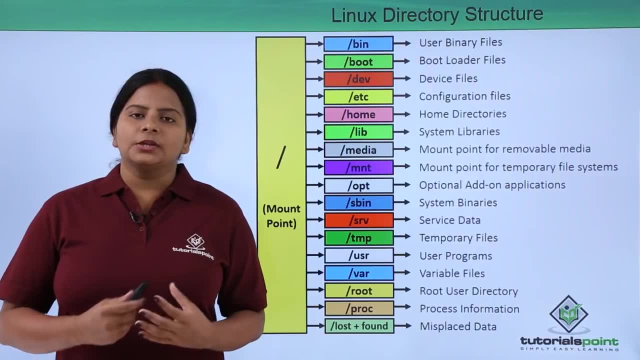 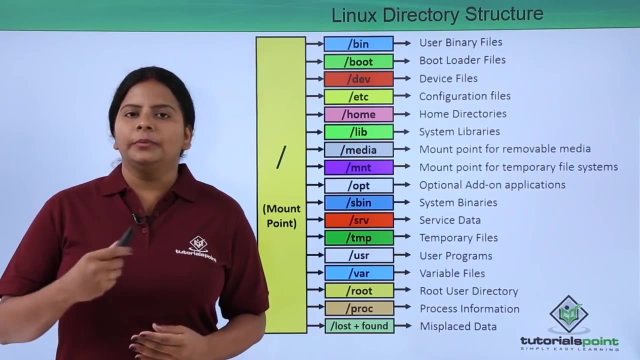 now, whatever the configuration you do, you define a host name, you define IP address, you configure some servers like your FTP particular servers, all this particular services, all this particular settings will be stored under slash, etc. so, whichever the configuration is, all the configuration file you will be finding into slash, etc. the next directory which 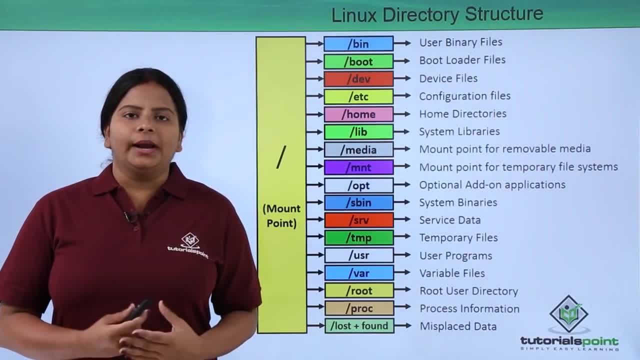 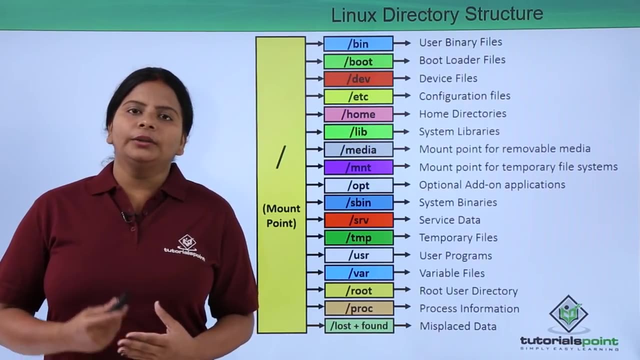 we have that is slash home. so slash home is a directory which contains the home directory of your users. now we can see multiple users or we can create multiple users into the Linux operating systems. so when this users get login, all the data which they are going to create on their desktops, on their documents or any, 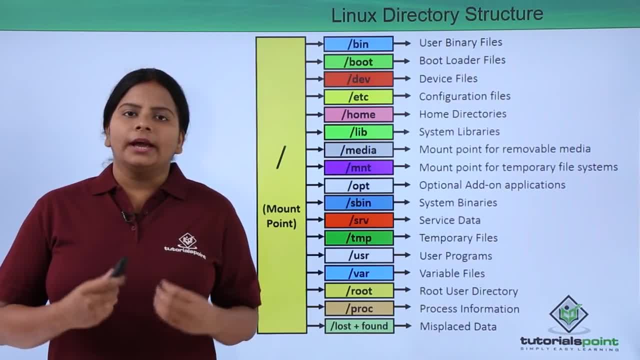 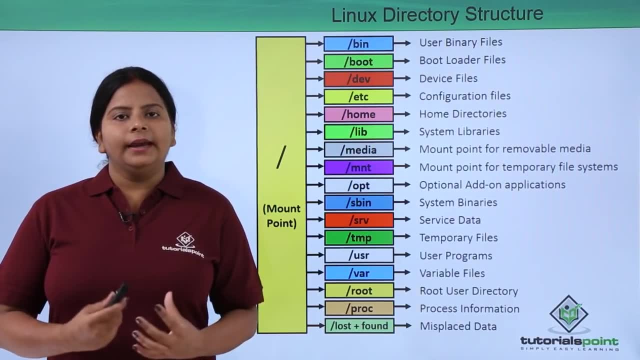 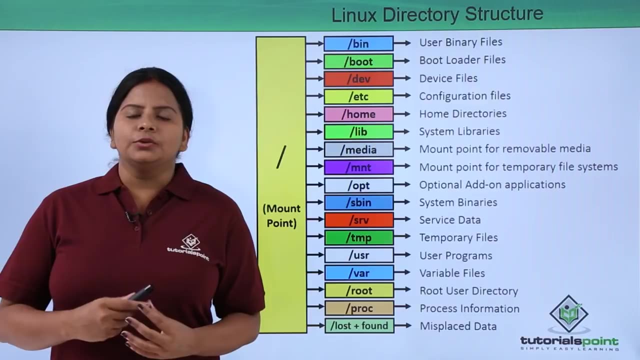 of their directories. all this will be created and saved into this slash home directory. so if suppose I have created a user with name user 1, so the home directory will create a separate folder for user 1 and whenever the user will log in, this particular data of this user 1 will be stored into slash home slash. 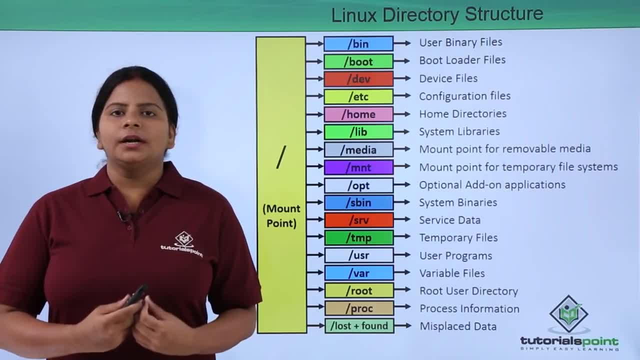 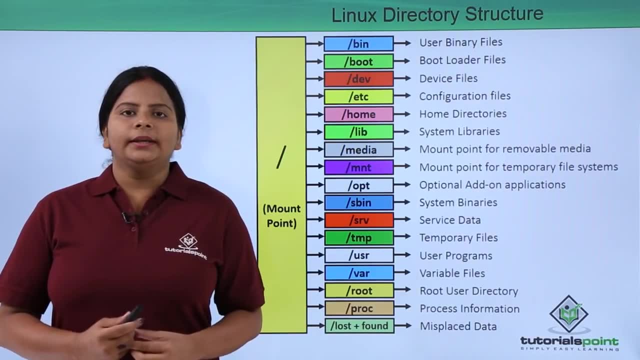 user 1 directory. so same way for other user, like your user 2, it will create a another directory, so none of the user will be able to see each other's data. that generally is stored into the home but is basically only for your standard users, which is a non root or non super users. next directory which we have: that 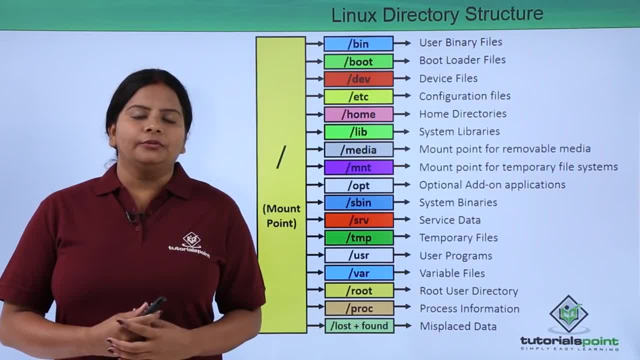 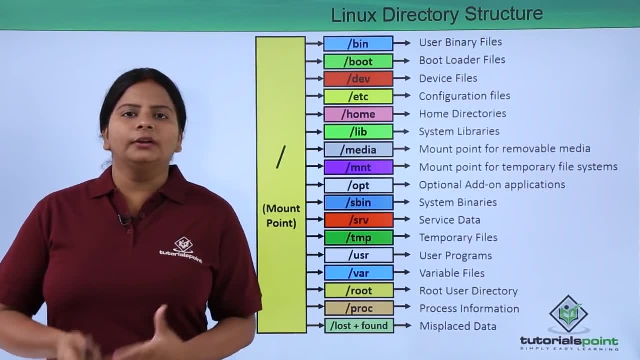 is slash lib, so lib contains all the library files. now, if suppose you want some help, if you want to get some help regarding any particular command or how to configure that particular command, or you can see the parameters, what the parameters we have for a particular command, all the help. 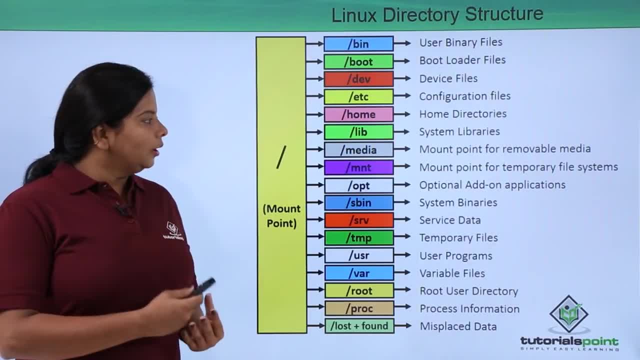 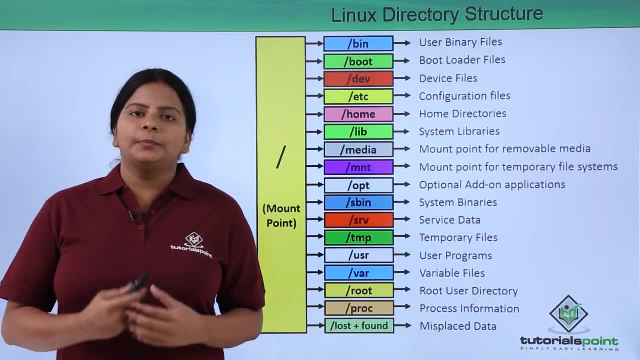 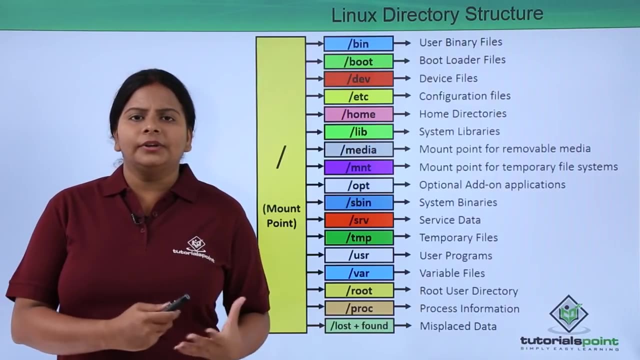 option you get into the library. the next we have that is called as a slash media. so slash media is basically a directory created so that you can find this particular hot plug-and-play device is auto mounted over here now. basically, in previous organization we never used to have the slash media, but now we have the. 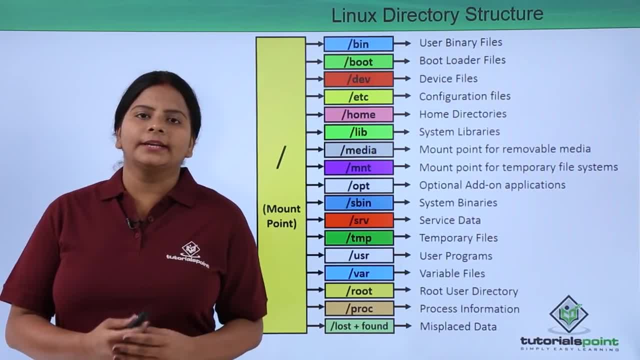 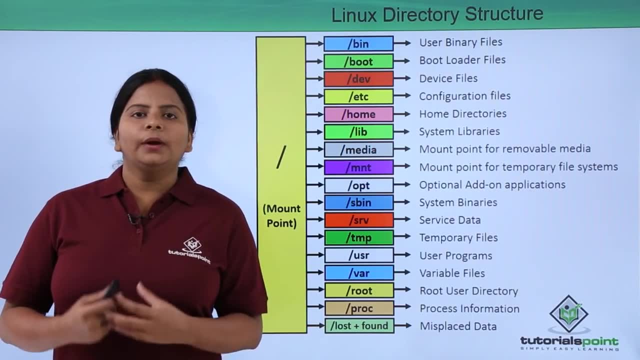 slash media so that it is easier for the users to work on the desktop of any of the Linux distributors, so that if they connect any hard pluggable device like your USB or you connect a DVD drive directly, it will be mounted on your desktop. means if you. 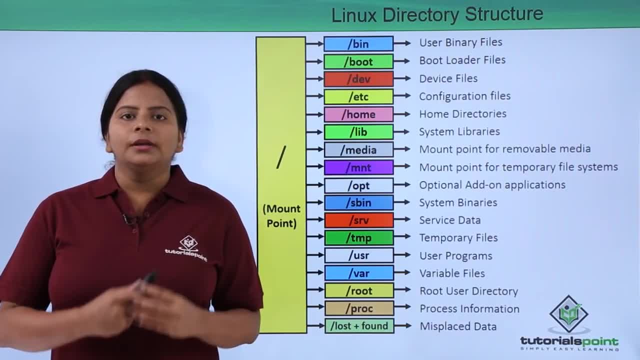 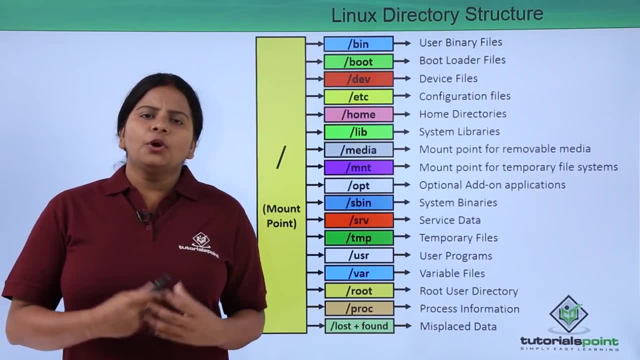 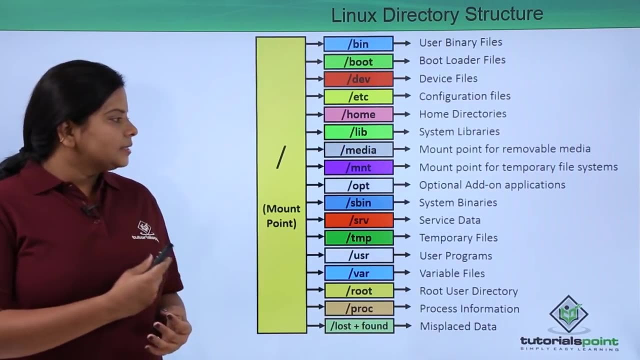 will be seeing it on your desktop because it is by default stored and located into slash media directory. next we have that is slash opt, so all the optimized data is whatever you have that will be stored into these slash opt. next we have that is called as a slash pin, so slash 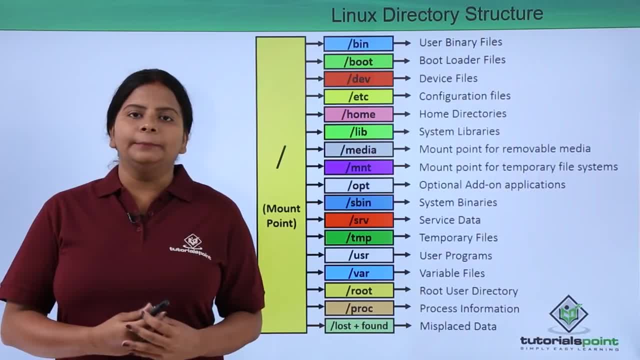 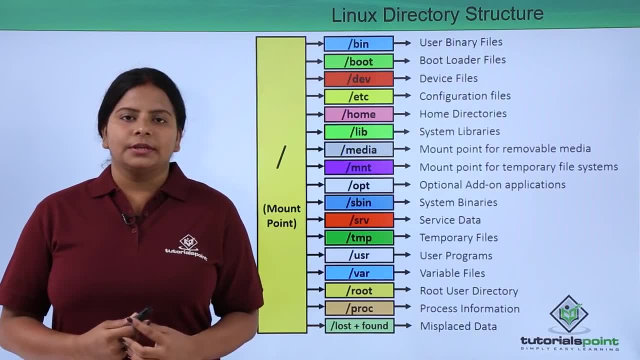 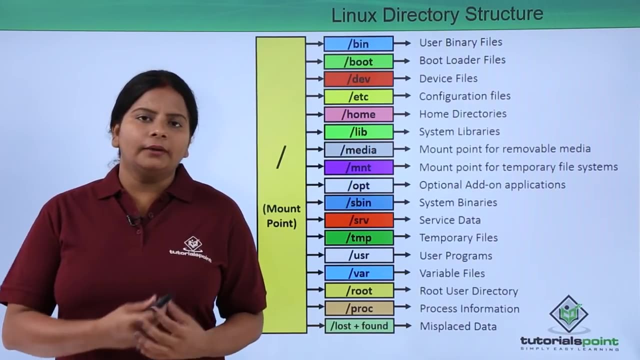 is a super win. now, earlier we had discussed about the bin, where I have told you it contains all the binary files, but this binary files are only for the standard users, like if I want to create a new user using a particular standard user, I won't be able to do that, even you have the same thing into. 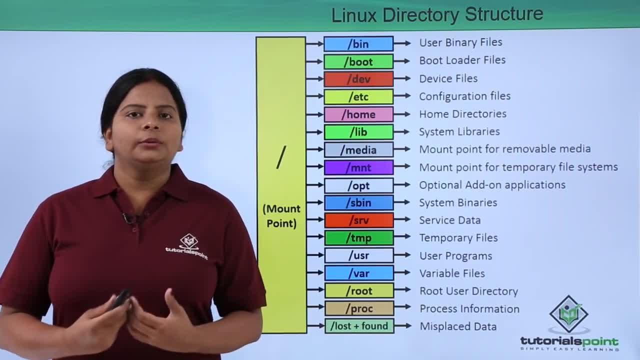 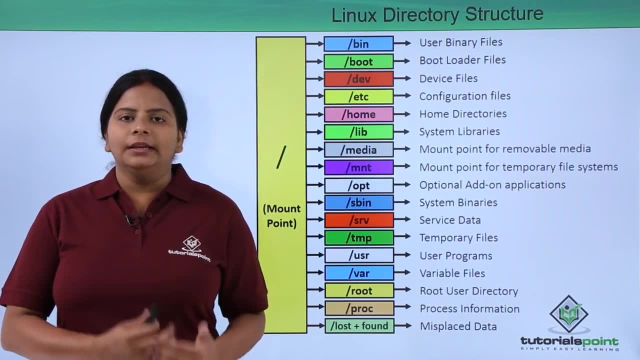 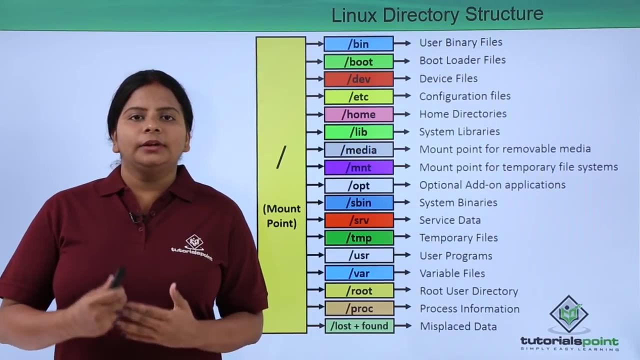 Windows operating system right from a standard user. you cannot create a new user because it's completely command are stored into different location, even in Windows and even in the Linux operating system. so basically, when the basic user or we can see a standard users get login, they generally access slash bin. but what if? about your super user? super user is 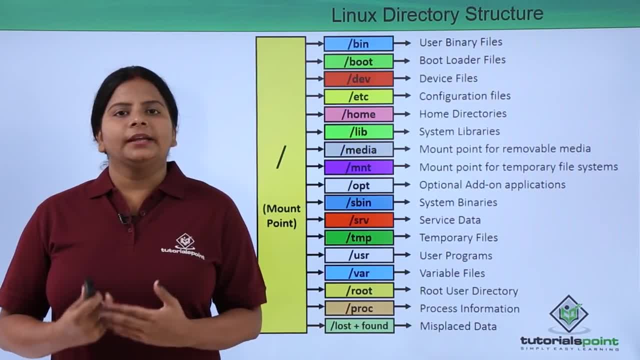 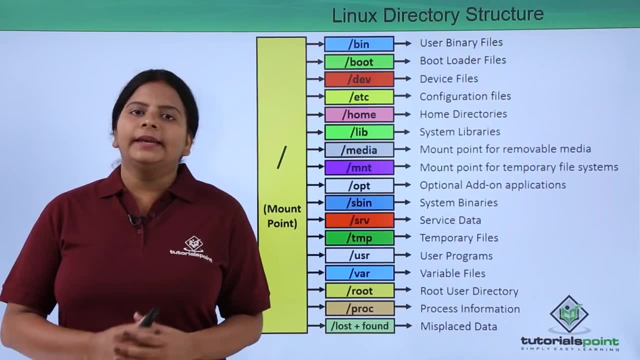 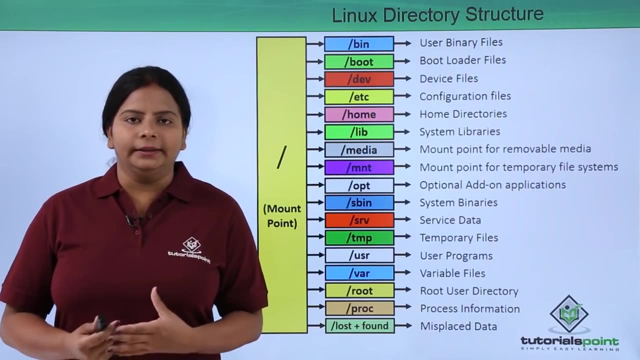 nothing but a root user. root user is just like an administrator you have into the windows. so this particular user, root user, have access to everything. he can do everything into the Linux operating system. he can modify anything, he can create anything, he can configure anything or delete anything. so this: 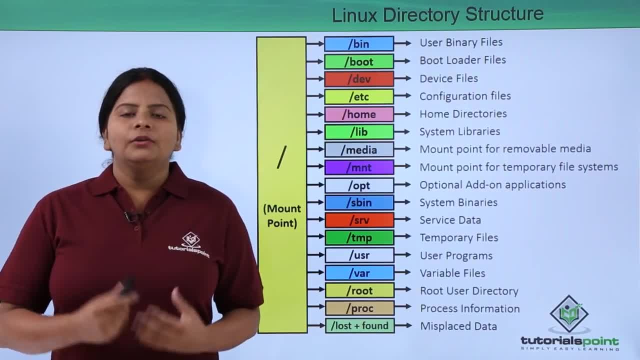 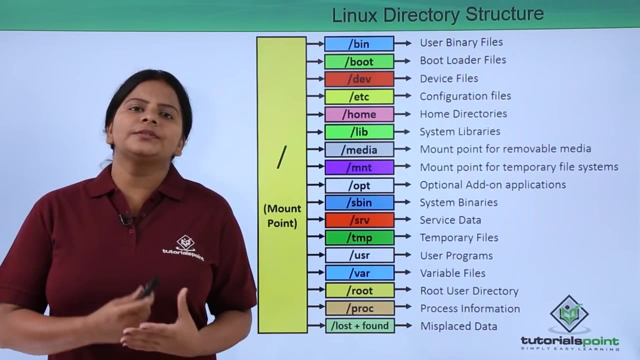 super user use this slash as bin for storing. it's all. the particular binary file and what are the commands is going to use will be pulled by this particular binary folder itself. the next we have that is called as a slash SRV, so all the service related data with services are on which services are started on the. 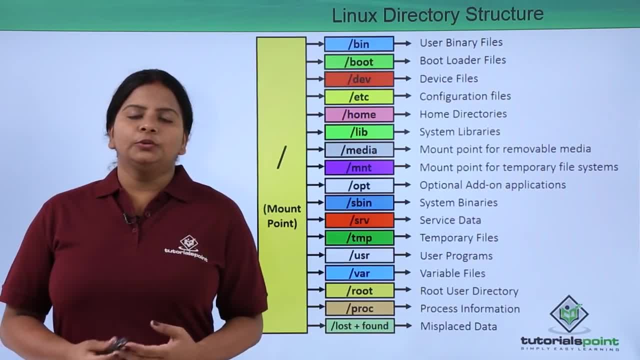 boot or with services are stopped. all this particular data you will find into slash SRV. the next directory which we will use is this: slash S which is a. the next directory which we will use is this: slash S, which is a, slash S which is a, which we have. that is your slash temp. you may be knowing about the temp directory, so if suppose 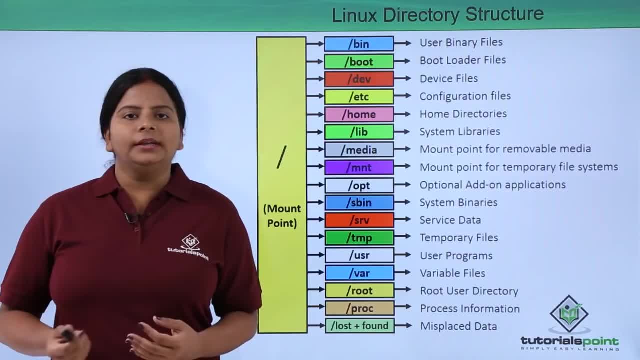 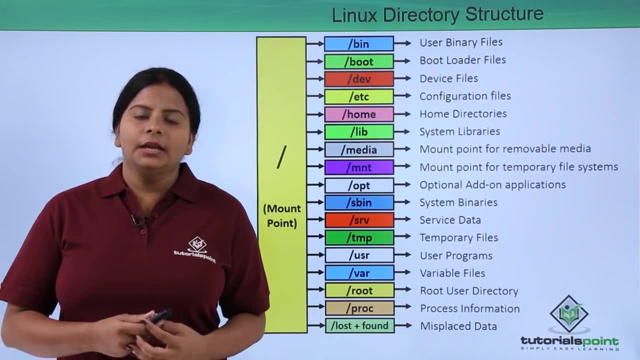 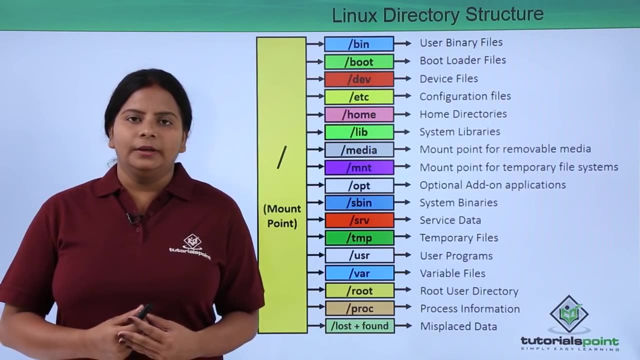 you are doing some temporary task, like you are copying a dvd from one drive to your hard disk or you are creating a dvd dvd images, correct? so if you are using the dvd dvd image, it temporarily stores the data into your ram for a particular period of time, so that it stores into this slash. 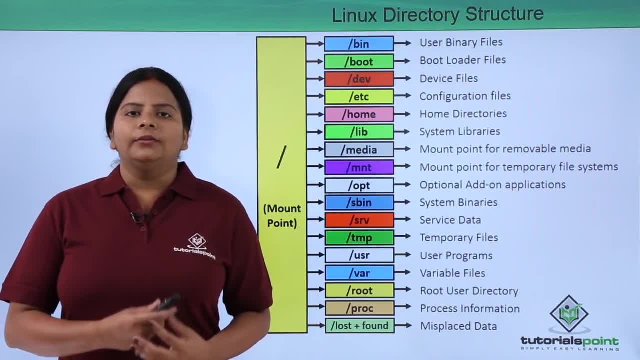 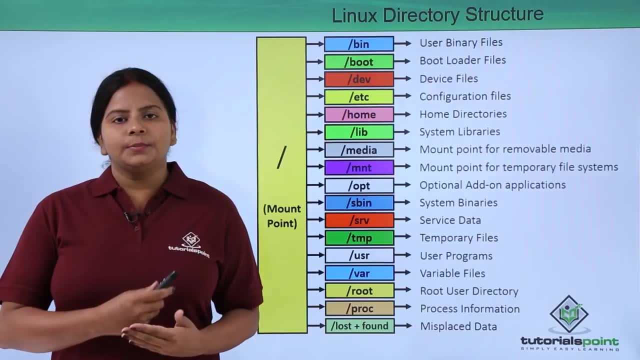 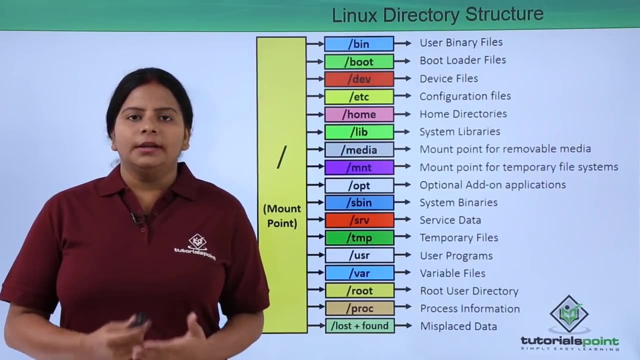 temp folder into your windows, and here we have a slash temp. so whatever the temporary files you want you can store into the temp. once your system is rebooted, this particular files will get flushed out. so that's the reason they are called as a volatile storage for your linux operating system. 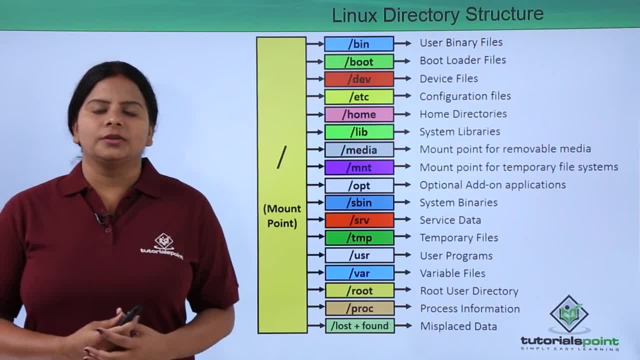 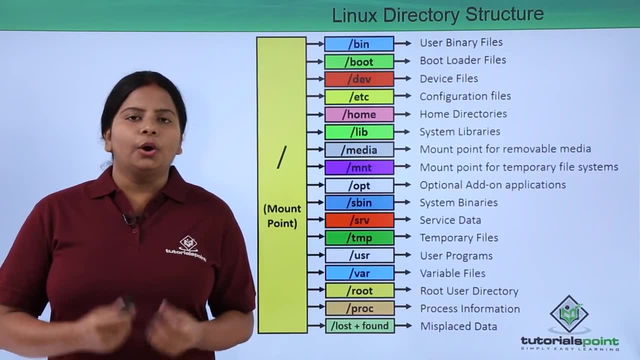 the next directory which we have, that is, your slash usr. so slash usr contains all the user programs. now, for example, you have installed some package or you have downloaded some package, or you have downloaded some program into your linux operating system, all the particular files of that particular program will be stored into slash usr. this usr will create all the samples files of 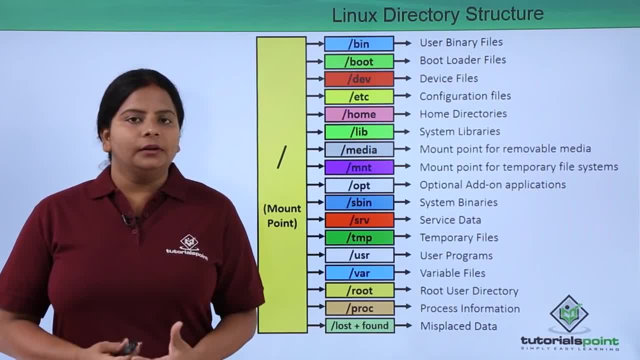 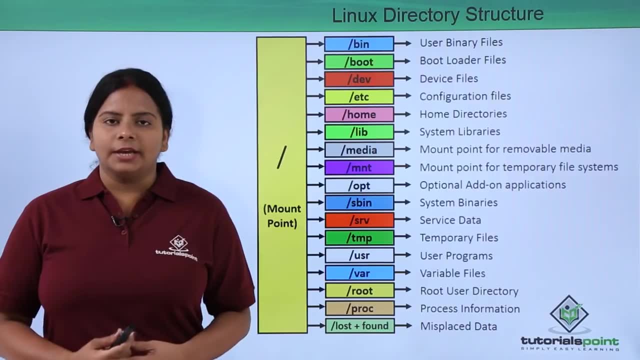 that particular program. so if suppose you do not know how to configure particular server or particular program, you will be having those particular sample files pre-configured into the slash usr. you can get the data, you can copy those particular files into slash, etc. where we keep all. 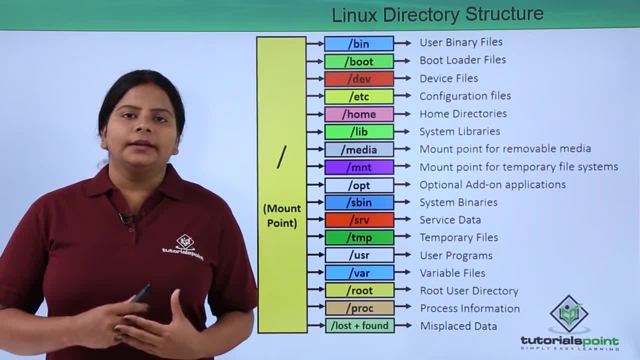 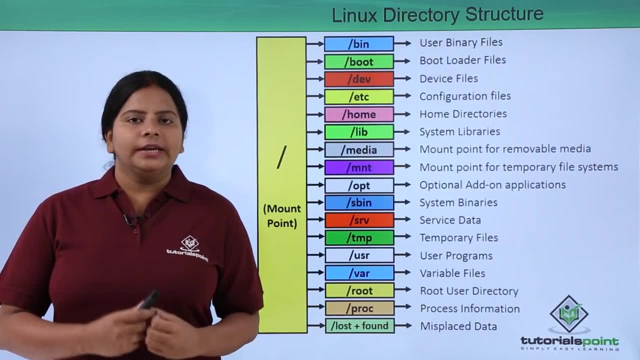 the configuration and configure it. so slash usr contains all the particular programs, applications, tools and the services which you've installed. data will be stored into it. the next directory which we have, that is your slash var. it contain all the variable files. so, basically, what are variable files? 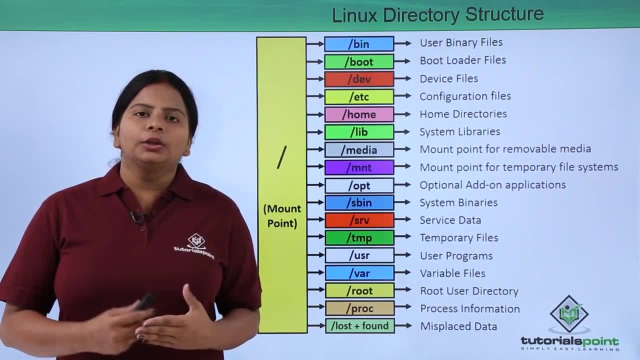 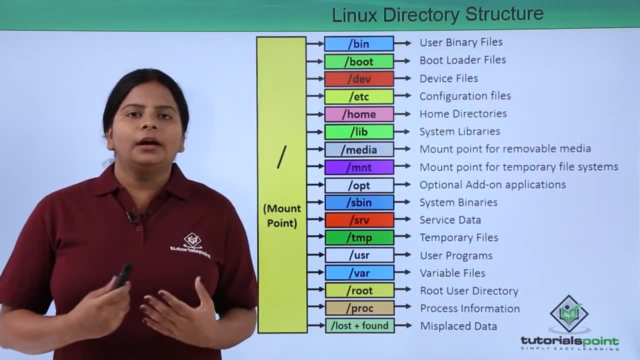 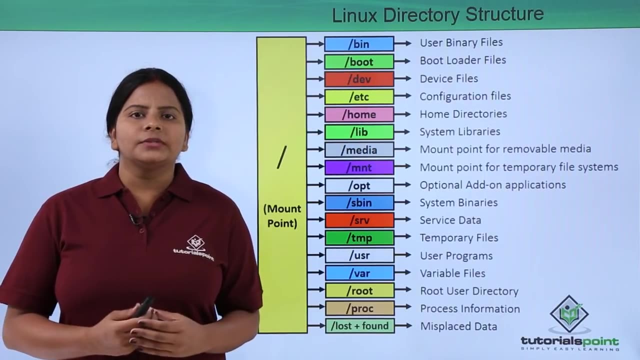 variable files or variable datas are those things which generally change. like, for example, i can say: you have defined an ip address to your machine on a dynamic way. so dynamic way means it is going to change whenever the server releases this particular ip address. so you might have seen, when you connect your wireless devices, your ip changes. 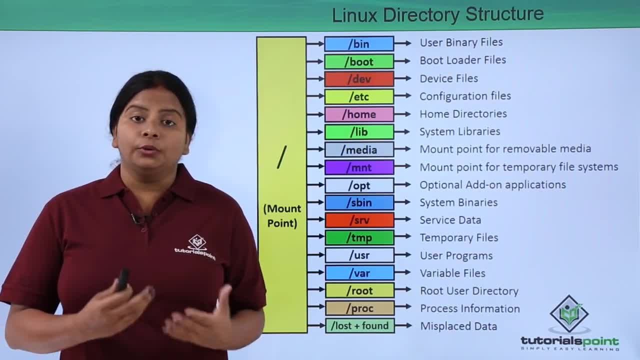 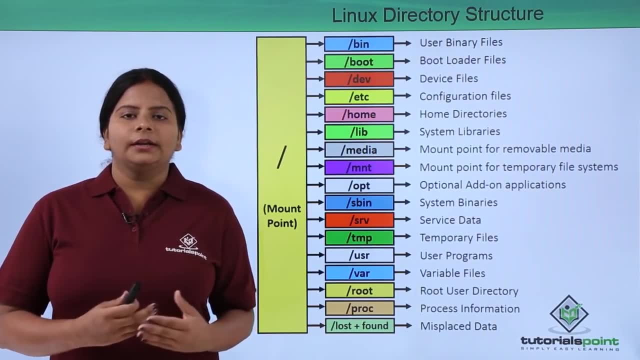 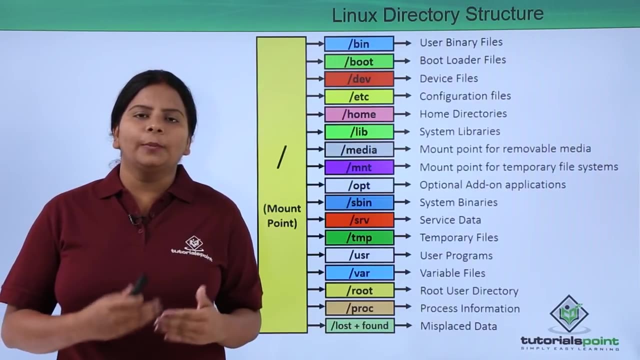 same way, if you might, you can see about your dns, if you know about dns. dns is a domain name system. it contains all the host name of all the particular systems which are connected into a particular domain. so if a domain name changes or if your ip address of your local host changes it automatically. 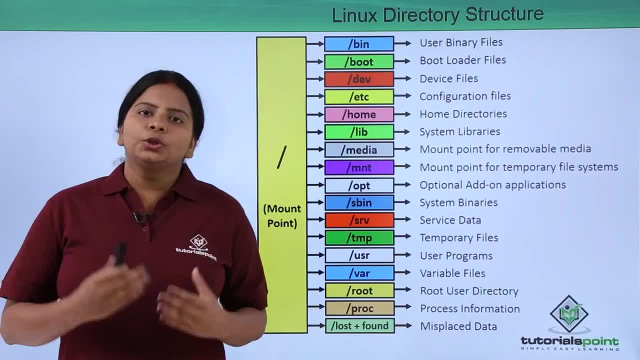 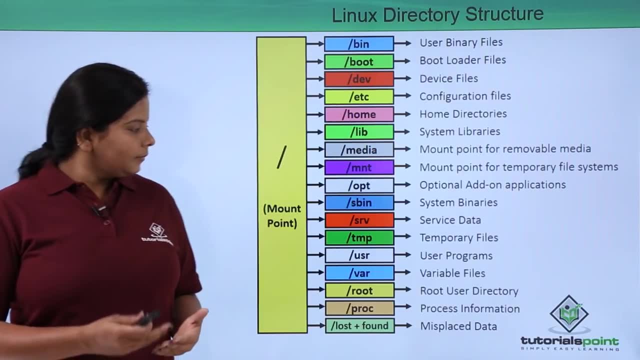 replicate or change the domain name of your system. so if you connect your wireless devices to your network you will be able to change that into it. okay, so those datas which generally vary, which you know, which are not constant, are generally stored into slash var, the next directory which we have. 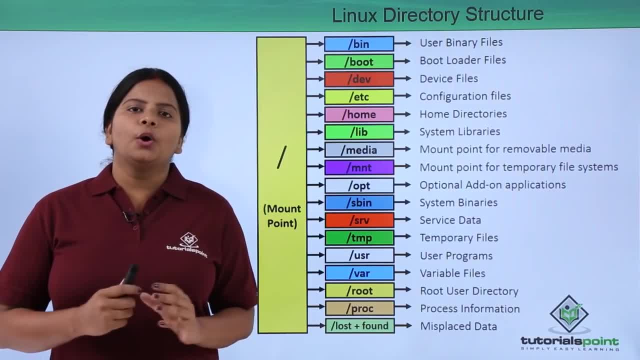 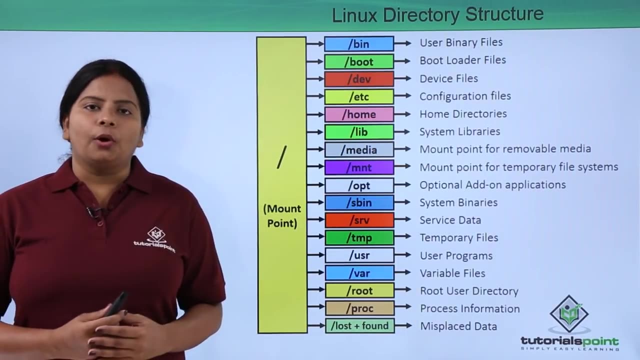 that is slash root. basically, slash root is a home directory of your super user root. slash home contains the standard user's home directory, but root stores its complete data into a different directory called as slash root. the next directory which we have slash frog. so this frog contains the. 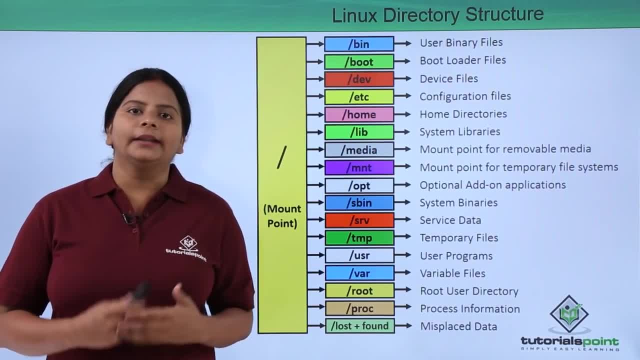 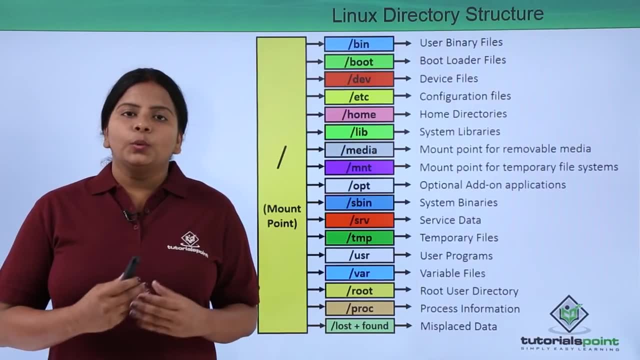 information about the devices you have connected and their process. now, for example, my memory which i have connected, that actually is used by your system, so we can see whether this memory is completely utilized or not. what is the process? what is the progress rate of the? you know the ram. 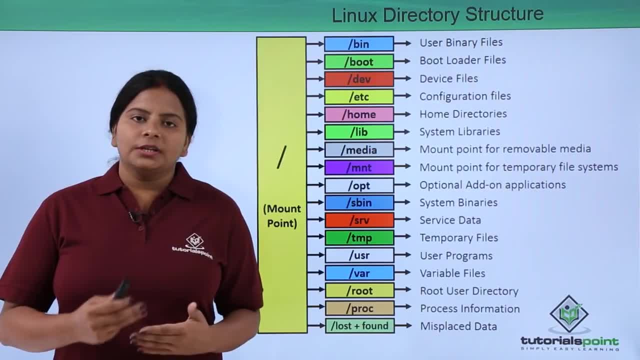 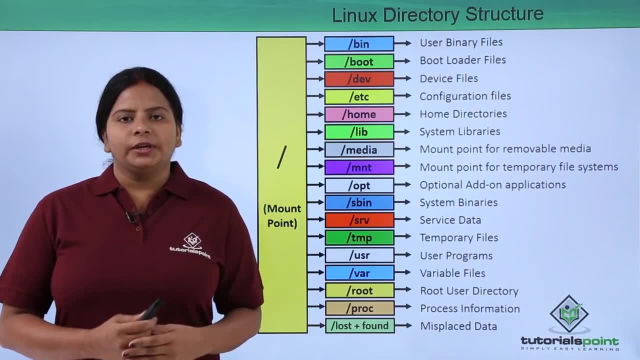 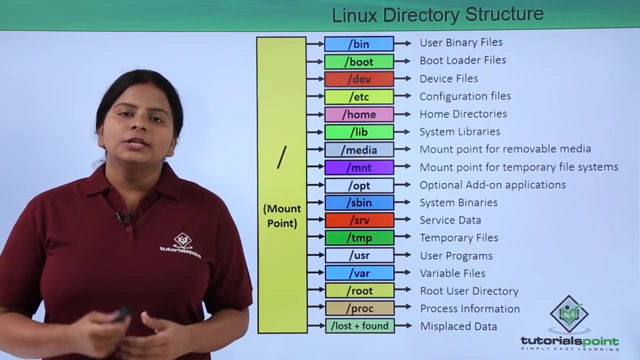 which we are using, what is the service which we are using, what is the progress rate of it, what is the utilization of your different devices, different resources connected to in the system. you can get all the information into slash frog. so basically, the last directory which we have that is called as a loss plus found. so loss plus found. 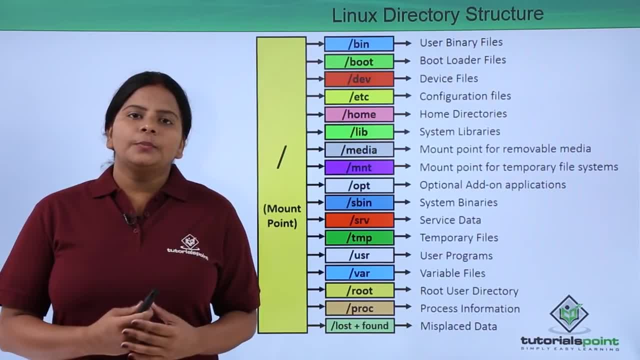 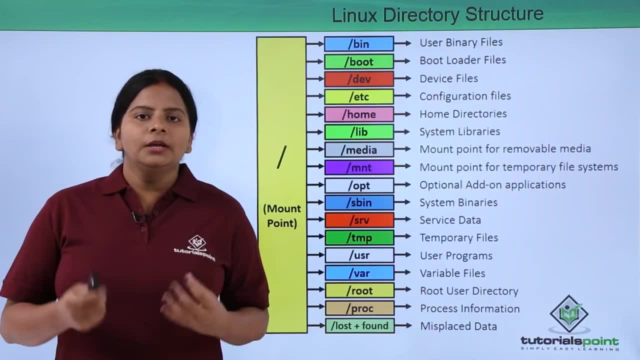 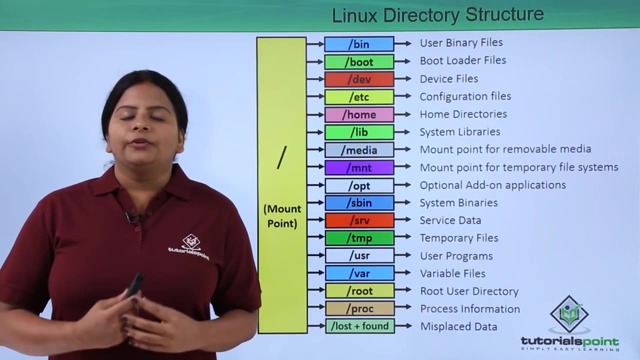 is a directory which we have into all the distributors. now this particular directory contains the data which is misplaced, like we do not have a proper location where it should be stored, so those particular data by default moves into your loss plus found. so this is the directory structure of your linux. now if i am going to add any device, i'll be adding into the day if i want.